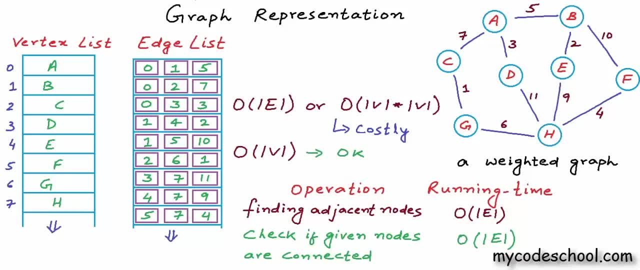 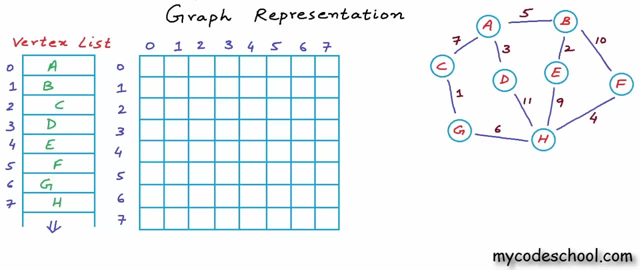 some other efficient design. We should think of something better than this. One more possible design is that we can store the edges in a two-dimensional array or matrix. We can have a two-dimensional matrix or array of size v, cross v, where v is number of vertices. As you can see, I have 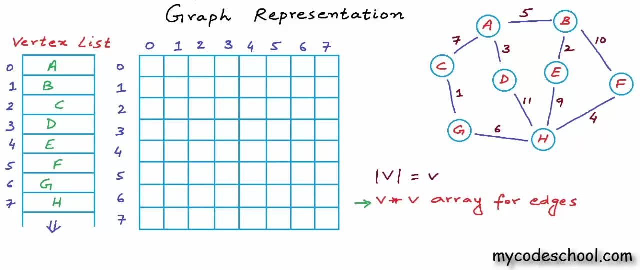 drawn an eight cross eight array here, because number of vertices in my example graph here is eight. Let's name this array a. Now, if we want to store a graph that is unweighted, let's just remove the weights from this example graph. here And now our graph is unweighted, And if we have a value or index between, 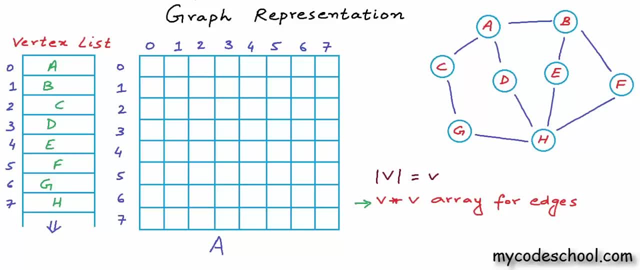 zero and v minus one for each vertex, which we have here. if we are storing the vertices in a vertex list, then we have an index between zero and v minus one For each vertex. we can say that a is zeroth node, b is oneth node, c is twoth node, and so on. 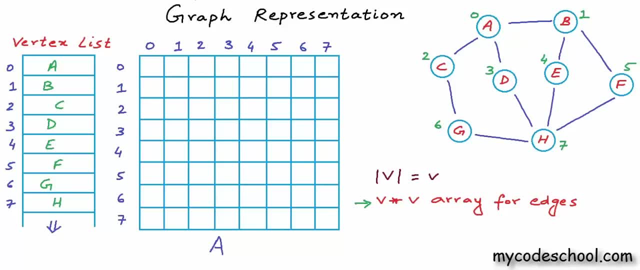 We are picking up indices from the vertex list. Okay, so if the graph is unweighted and each vertex has an index between zero and v minus one, then in this matrix or 2D array, we can set i-th row and j-th column. that is, a, i, j. 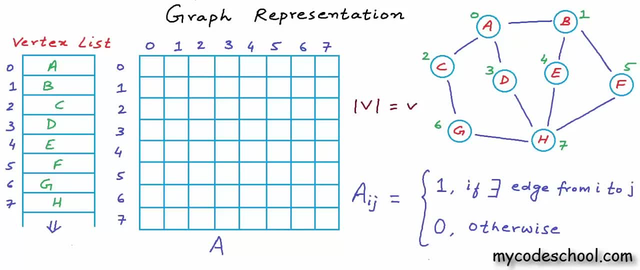 As one or boolean value, true if there is an edge from i to j, zero or false. otherwise, If I have to fill this matrix for this example graph here, then I'll go vertex by vertex. Vertex zero is connected to vertex one, two and three. Vertex one is connected to zero, four and five. 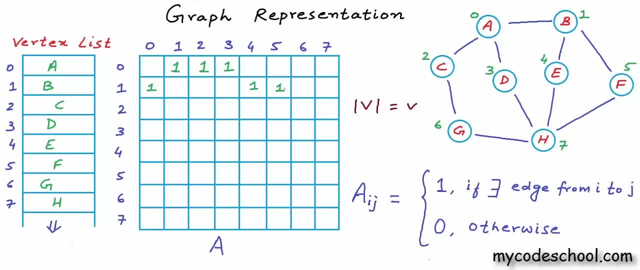 This is an undirected graph. This is an undirected graph. This is an undirected graph. So if we have an edge from zero to one, we also have an edge from one to zero. So oneth row and zeroth column should also be set as one. 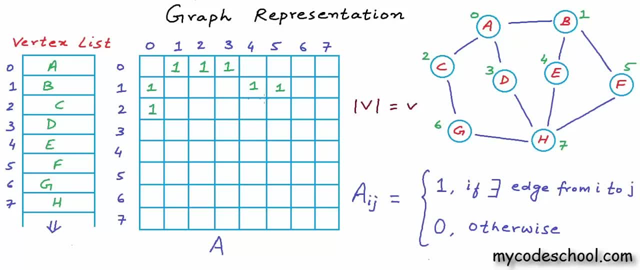 Now let's go to node two. It's connected to zero and six. Three is connected to zero and seven. Four is connected to one and seven. Five, once again, is connected to one and seven. Six is connected to two and seven. 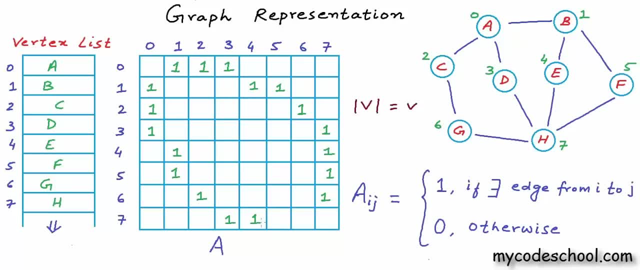 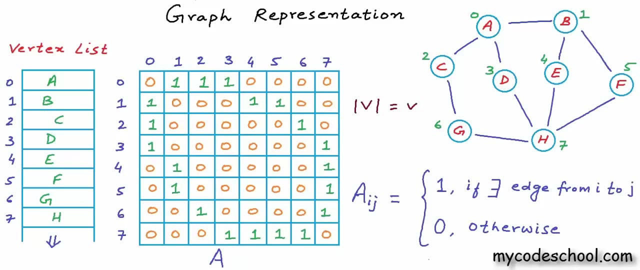 Seven is connected to three, four, five and six. All the remaining positions in this array should be set as zero. Notice that this matrix is symmetric. For an undirected graph, this matrix would be symmetric Because a i- j would be equal to a j- i. 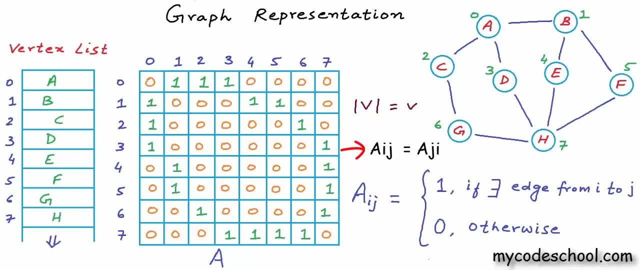 We would have two positions filled for each edge. In fact, to see all the edges in the graph, we need to go through only one of these two halves. Now, this would not be true for a directed graph. Only one position will be filled for each edge. 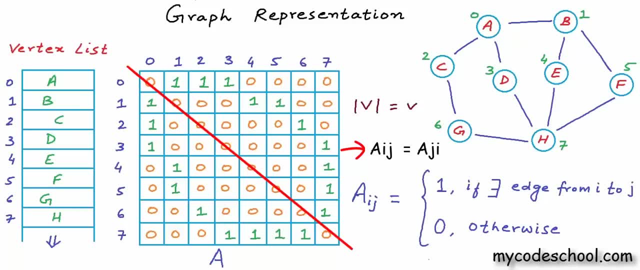 and we will have to go through the entire matrix to see all the edges. Now, this kind of representation of a graph in which edges or connections are stored in a matrix or 2D array is called adjacency matrix. This particular matrix that I have drawn here is an adjacency matrix. 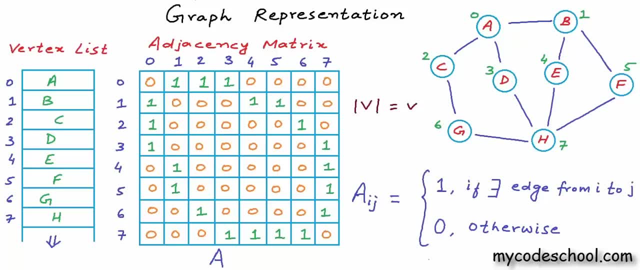 Now, with this kind of storage or representation, what do you think would be the time cost of finding all nodes adjacent to a given node? Let's say, given this vertex list and adjacency matrix, we want to find all nodes adjacent to node named F. 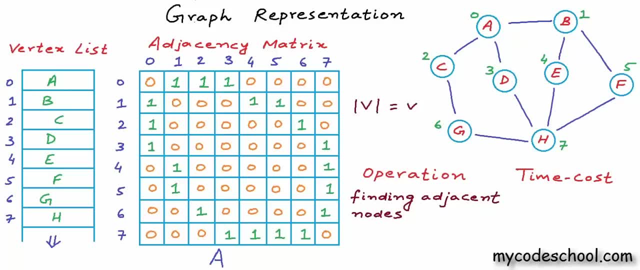 If we are given name of a node, then we first need to know its name, Then we need to know its index. And to know the index we will have to scan the vertex list. There is no other way. Once we figure out the index, like for F. 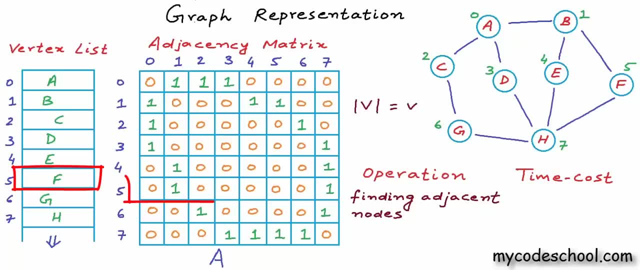 index is 5, then we can go to the row with that index in the adjacency matrix and we can scan this complete row to find all the adjacent nodes. Scanning the vertex list to figure out the index in worst case will cost us time proportional. 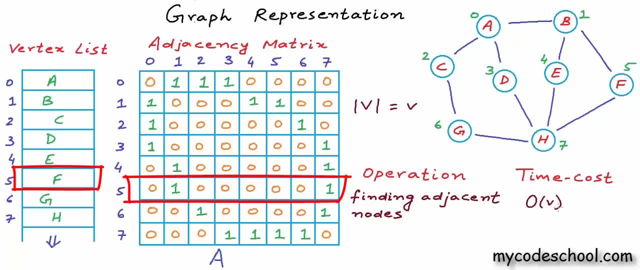 to the number of vertices, Because in worst case we may have to scan the whole list And scanning a row in the adjacency matrix would once again cost us time proportional to number of vertices, because in a row we would have exactly V columns where V is number of vertices. 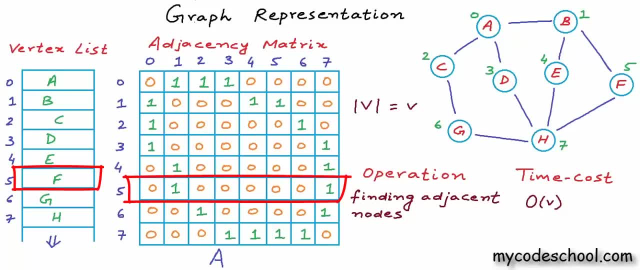 So overall time cost of this operation is O. Now, most of the time while performing operations we must pass indices to avoid scanning the vertex list all the time. If we know an index, we can figure out the name in constant time. 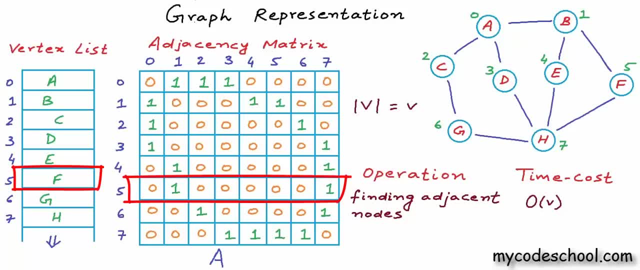 Because in an array we can access element at any index in constant time. But if we know a name and want to figure out the index, then it will cost us big O. We will have to scan the vertex list. We will have to perform a linear search on it. 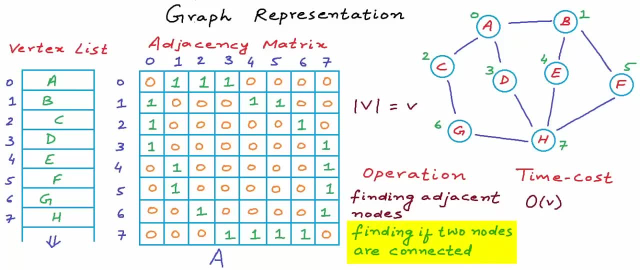 Okay, moving on Now. what would be the time cost of finding if two nodes are connected or not? Now, once again, the two nodes can be given to us as indices or names. If the nodes would be passed as indices, then we simply need to look at value. 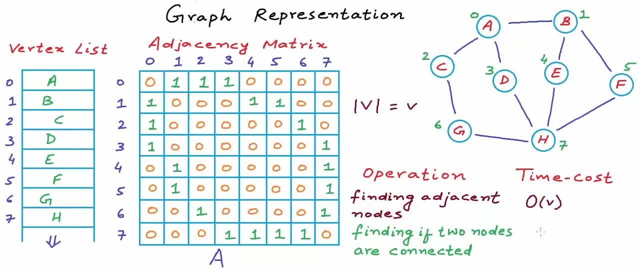 in a particular row and particular column. We simply need to look at aij for some values of i and j And this will cost us constant time. You can look at value in any cell in a two-dimensional array for constant time. So if indices are given, 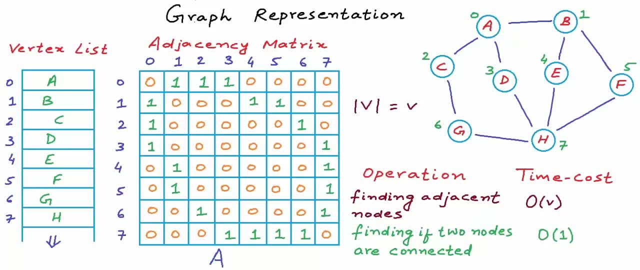 time complexity of this operation would be big O, which simply means that we will take constant time. But if names are given, then we also need to do the scanning to figure out the indices, which will cost us big O. Overall time complexity would be big O. 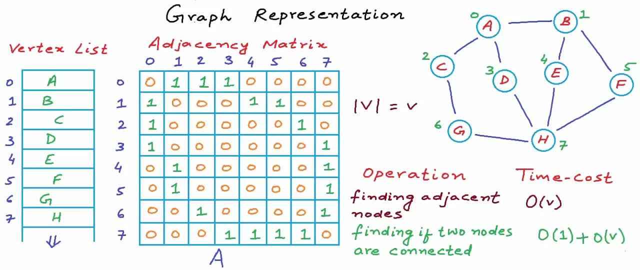 The constant time axis would not mean anything. The scanning of vertex list all the time to figure out the indices can be avoided. We can use some extra memory to create a hash table with names and indices as key value pairs. And then the time cost of finding index from name. 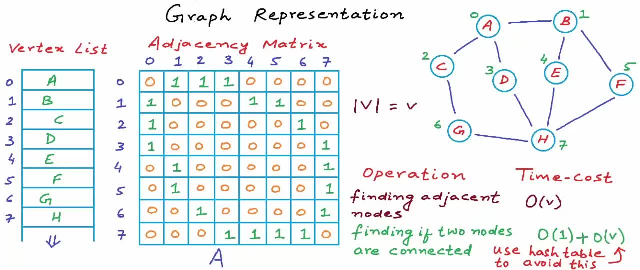 would also be big O, that is constant. Hash table is a data structure and I have not talked about it in any of my lessons so far. If you do not know about hash table, just search online for a basic idea of it. Ok, so, as you can see, 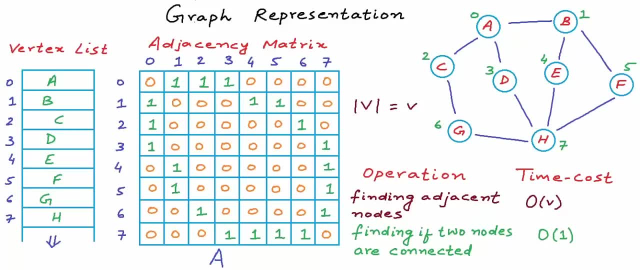 with adjacency matrix representation. our time cost of some of the most frequently performed operations is in order of number of vertices and not in order of number of edges, which can be as high as square of number of vertices. Ok, now if we want to store a weighted graph. 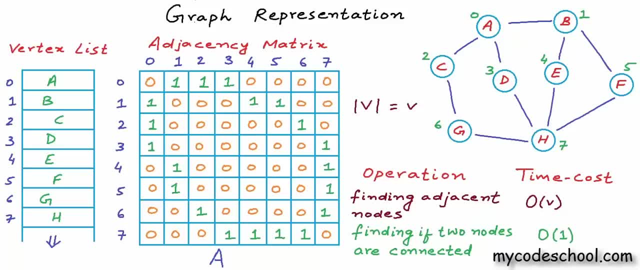 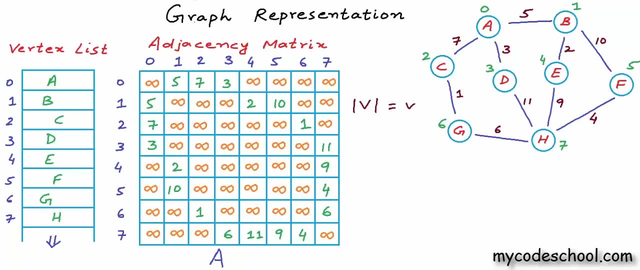 in adjacency matrix representation, then aij in the matrix can be set as weight of an edge. For non-existent edges we can have a default value like a really large or maximum possible integer value that is never expected to be an edge weight. I have just filled in infinity here. 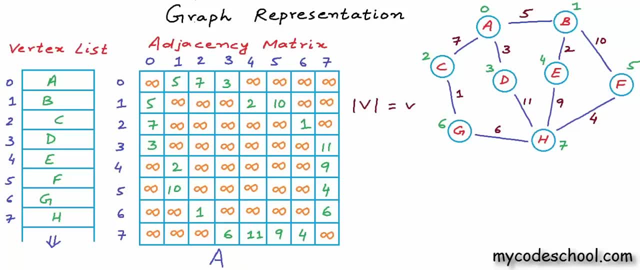 to mean that We can choose the default as infinity minus infinity or any other value. that would never, ever be a valid edge weight. Ok, now for further discussion. I will come back to an underlying non-weighted graph. Adjacency matrix looks really good. 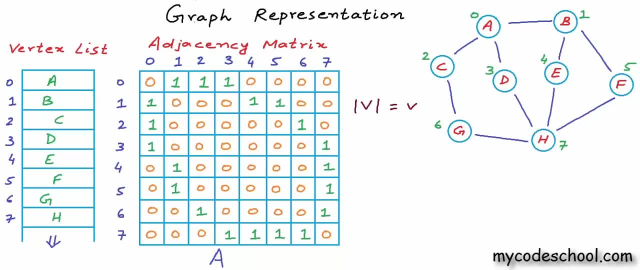 so should we not use it always? Well, with this design we have improved on time, but we have gone really high on memory usage. Instead of using memory units exactly equal to number of edges, what we were doing with an edge list kind of storage. 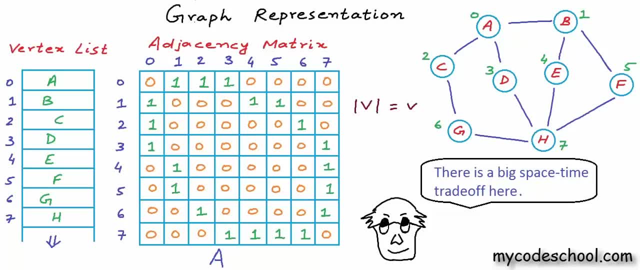 here we are using exactly v square units of memory. We are using big O of v square space. We are not just storing the information that these two nodes are connected, we are also storing not of it, that is, these two nodes are not connected. 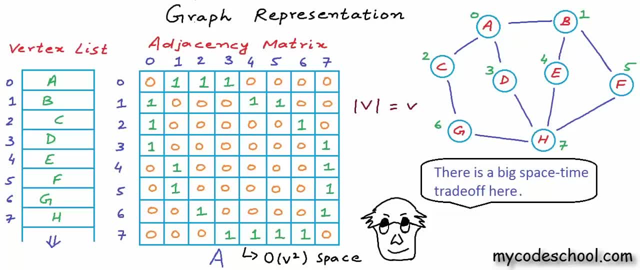 which probably is redundant information. If a graph is tense, if the number of edges is really close to v square, then this is good. but if the graph is sparse, that is, if number of edges is lot lesser than v square, then we are wasting a lot of memory. 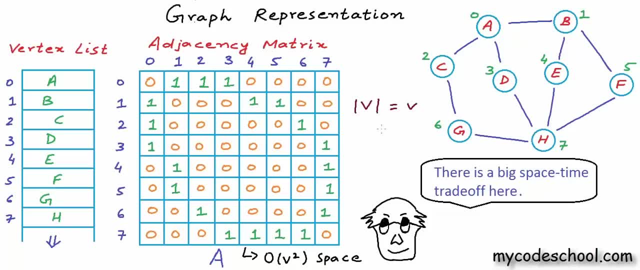 in storing these zeros, Like for this example graph that I have drawn here in the edge list, we were consuming 10 units of memory. We had 10 rows consumed in the edge list, but here we are consuming 64 units. Most graphs with 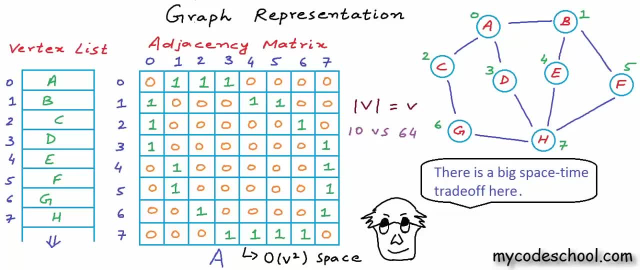 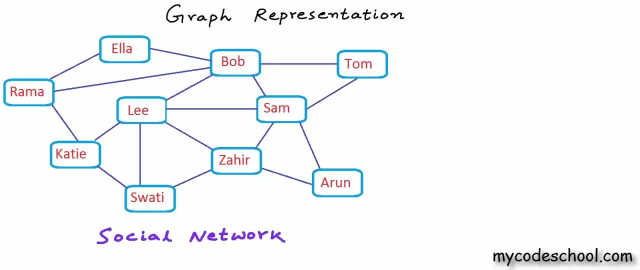 really large number of vertices would not be very tense, would not have number of edges anywhere close to v square, Like for example. let's say we are modeling a social network like Facebook as a graph, such that a user in the network is a node. 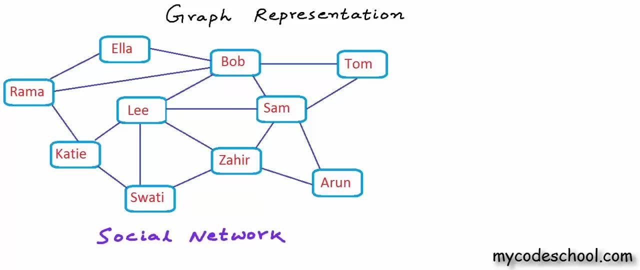 and there is an undirected edge if two users are friends. Facebook has a billion users, but I am showing only a few in my example graph here because I am short of space. Let's just assume that we have a billion users in our network. 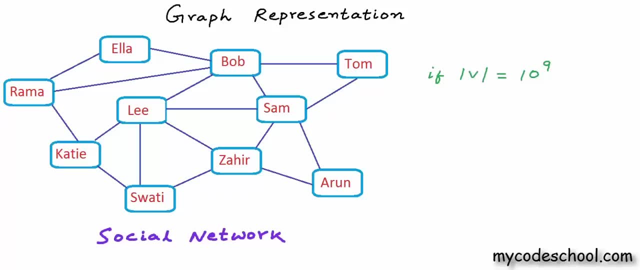 So number of vertices in our graph is 10 to the power 9,, which is a billion. Now do you think number of connections in our social network can ever be close to square of number of users? That will mean everyone in the network is a friend of everyone else. 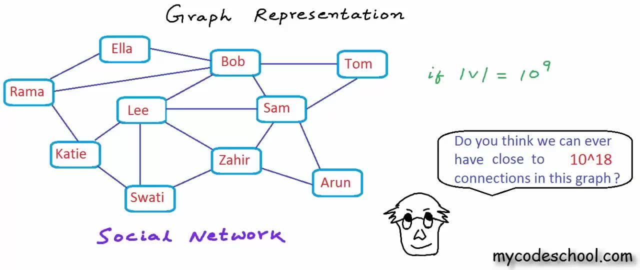 A user of our social network will not be friend to all other billion users. We can safely assume that a user, on an average, would not have more than a thousand friends. With this assumption, we would have 10 to the power, 12 edges in our graph. 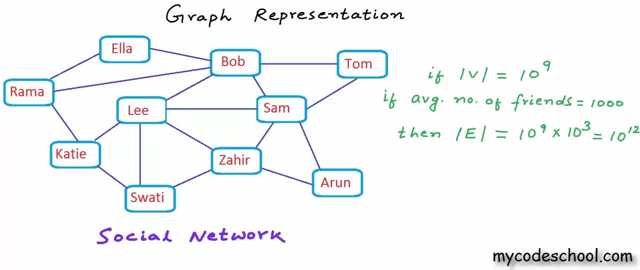 Actually this is an undirected graph, so we should do a divide by 2 here so that we do not count an edge twice. So if average number of friends is 1000, then total number of connections in my graph is 5 into 10 to the power 11.. 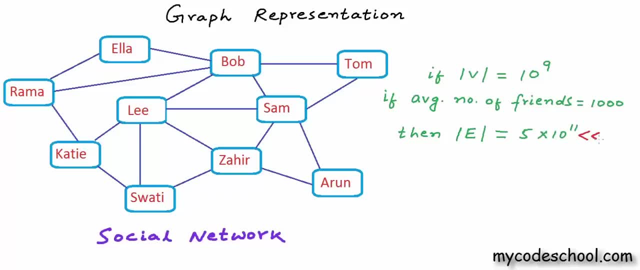 Now this is a lot lesser than square of number of vertices. So, basically, if we would use an adjacency matrix for this kind of a graph, we would waste a hell lot of space And, moreover, even if we are not looking in relative terms, 10 to the power, 18 units. 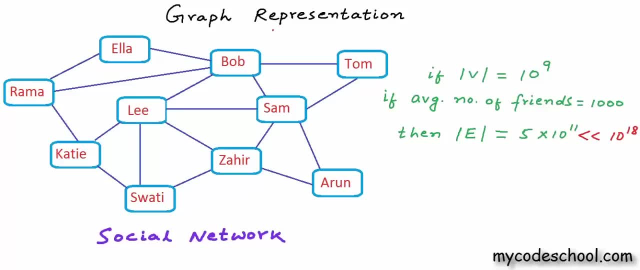 of memory, even in absolute sense, is a lot. 10 to the power, 18 bytes would be about a thousand petabytes. Now this really is a lot of space. This much data would never, ever fit on one physical disk. 5 into 10 to the power, 11 bytes. 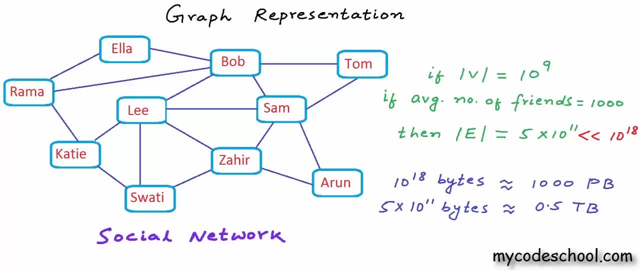 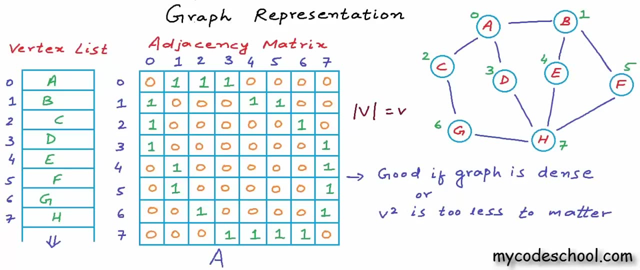 on the other hand, is just 0.5 terabytes. A typical personal computer these days would have this much of storage. So, as you can see, for something like a large social graph, adjacency matrix representation is not very efficient. Adjacency matrix is.